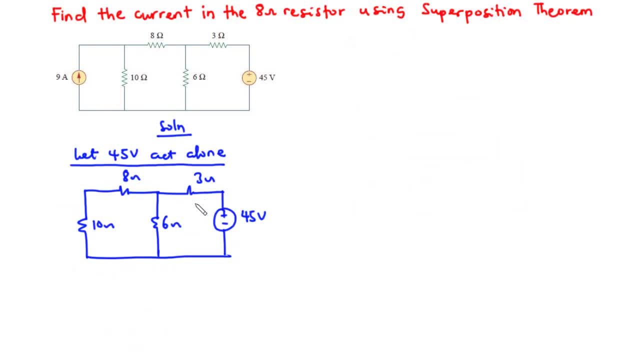 At this point, let's find the value of the total resistance for this circuit, so that we can find the current produced by this 45 volt, and then we can find the current flowing through the 8 ohms resistor when the 45 volt is acting alone. 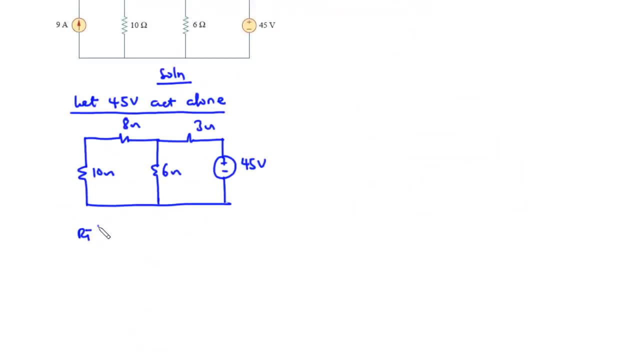 So let's call the total resistance for this circuit RT' and that is equal to Now. we have these two resistors connected in series because the same current will flow through them And the combination will be in parallel with a 6 ohms resistor. and all of that in series. 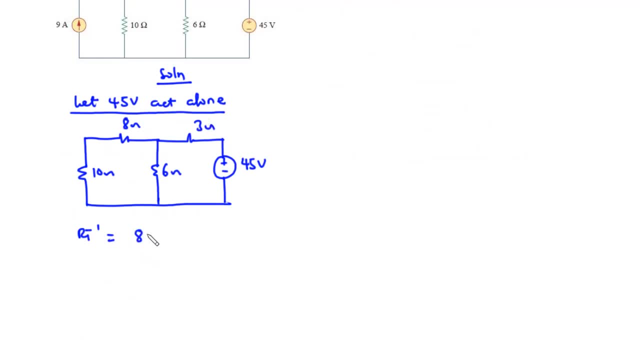 with a 3 ohms resistor. So we have 8 plus 10, or parallel 6, and all of that in series with a 3 ohms resistor, So plus 3.. So let's solve this. So we have 18 parallel 6, and that is equal to 18 times 6, divided by 18 plus 6 plus 3.. 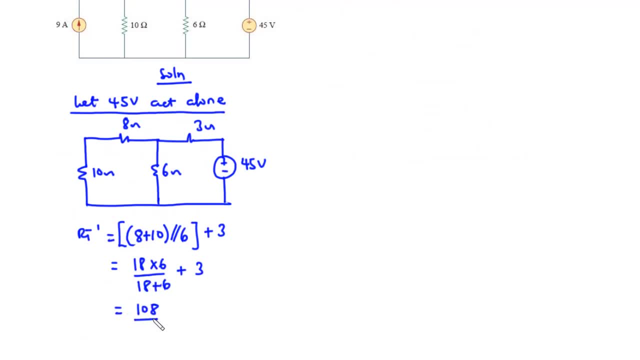 So 18 times 6. We have 108.. 18 plus 6, that is 24, and then we have plus 3.. Now this fraction, that is 108 divided by 24, gives 4.5, and then we have plus 3 and that. 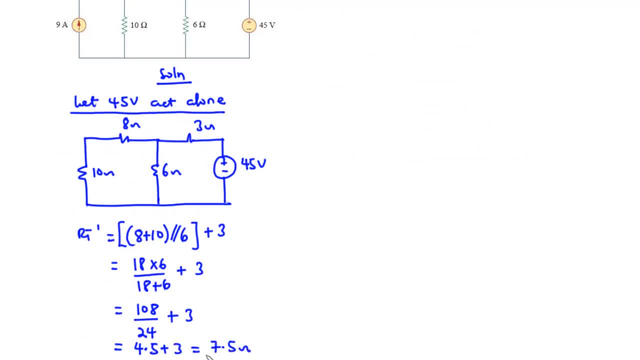 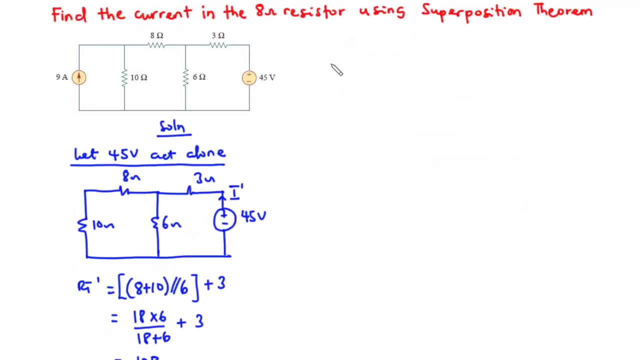 is equal to 7.5 ohms. So we have RT' to be 7.5 ohms. Now let's find the current produced by the 45 volts. Let's call that I'. So we have I' to be equal to Vain divided by RT'. that is, 45 divided by 7.5, and that is equal. 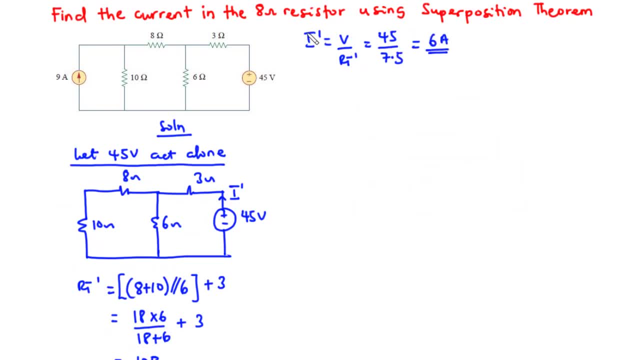 to 6 Amps. So we have the total current produced by the 45 volts to be 6 Amps. Now let's find the current that is going to flow through the 8 ohms resistor when the 45 volts are produced. 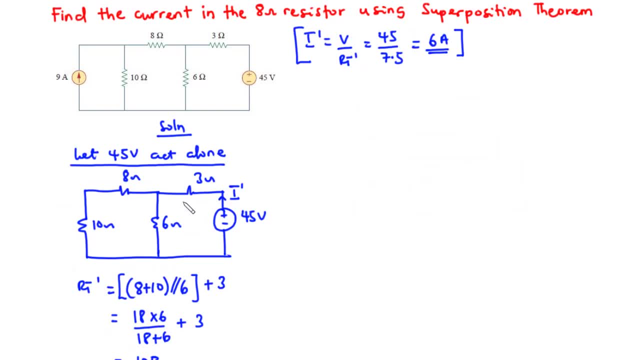 Let's call that I' 45V is acting alone, So this 6A current is going to flow in this direction, approaching this junction. Now, at this point, we can use the current division rule to find the current that is flowing in this branch, So the current that is going to flow through the 8 ohms resistor. 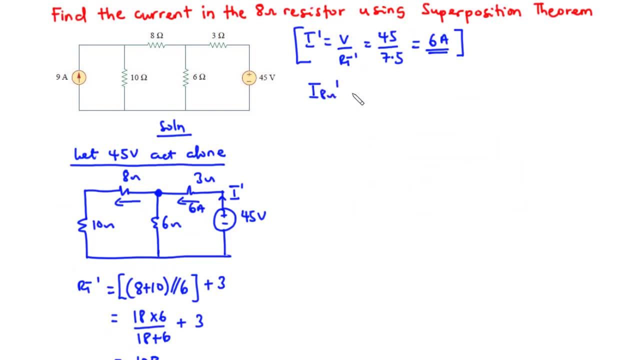 we can call that I8Ohm prime, and that is equal to the value of this resistor, which is 6 divided by. we are going to combine these two resistors Because we have the same current flowing through them, which means that they are connected in series. so that is going to be 18 and 6 divided. 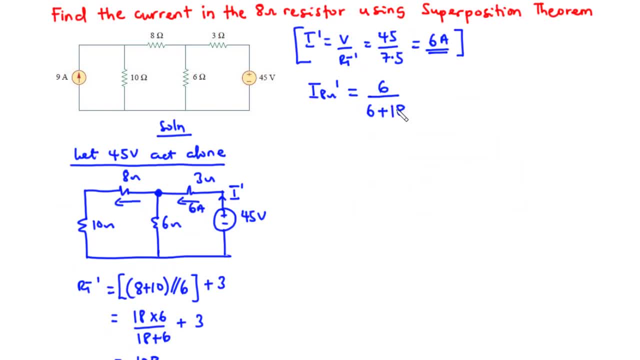 by 6 plus 18, using the current division rule. we are going to multiply that by the total current, the junction, which is 6 amperes. So when you solve this, you are going to get 1.5 amperes And notice the direction of the current. 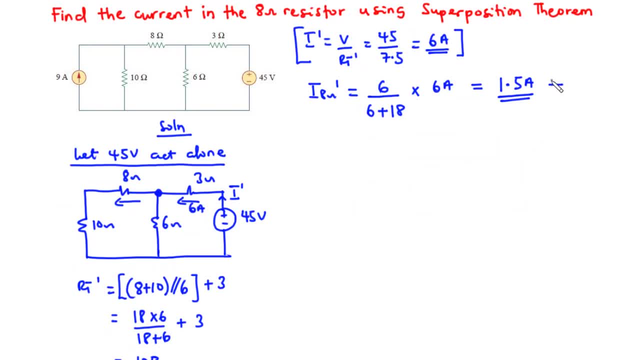 The current is moving this way, that is, to the left. So this is the direction of the current flowing through the 8 ohm resistor when the 45 volt is acting alone. Now, at this point, we are going to deactivate the 45 volts and then activate the 9 amperes. 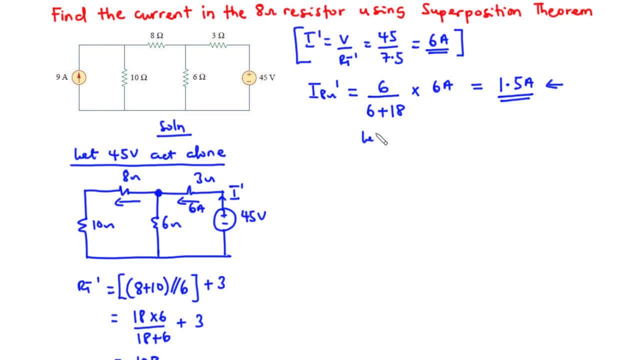 current. So let's do that. So let 9 amperes act alone. So let's redraw the circuit deactivating the 45 volts. So let's do that, So the 45 volts becomes a short circuit. We are going to represent that by a short circuit. 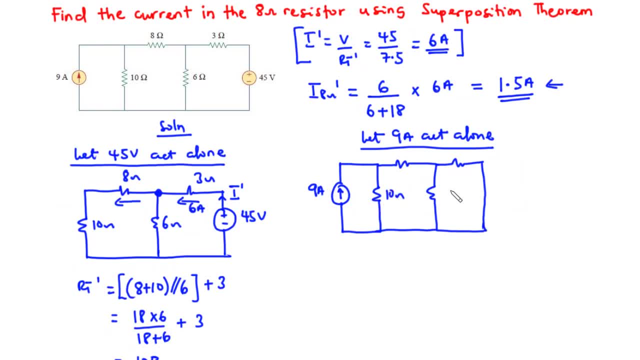 So that is that. So we have 10 ohms, 6 ohms, 3 ohms and then 8 ohms. So to find the current flowing through the 8 ohms resistor, first of all we need to combine these two resistors in parallel. 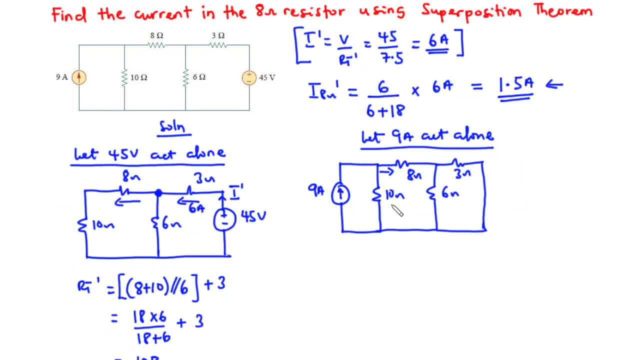 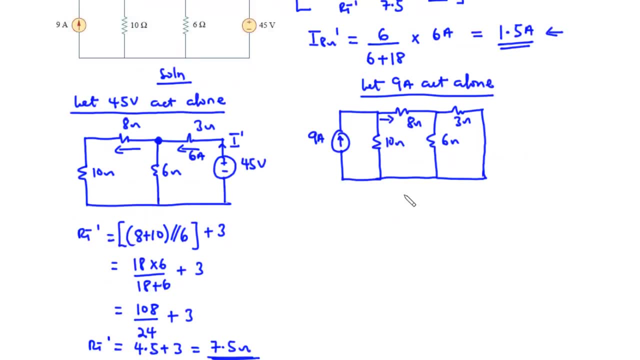 And then in series with this resistor, So that we can have two resistors and then we can distribute the current through them. So we can simplify this circuit, as we have the 9 amperes current And then we have this 10 ohms resistor. 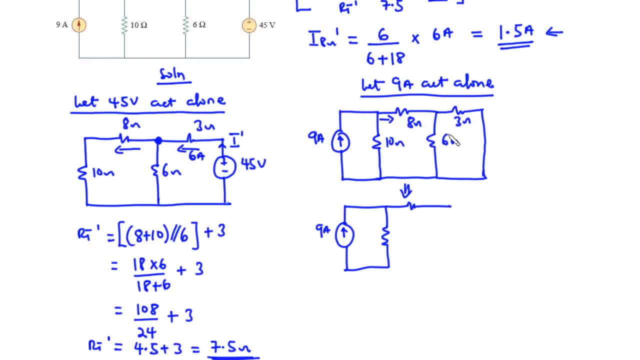 And then we have also the combination of these three resistors. Okay, Now let's find the combination of these three resistors. So we have 6 in parallel with the 3. So that is 6 times 3, divided by 6 plus 3.. 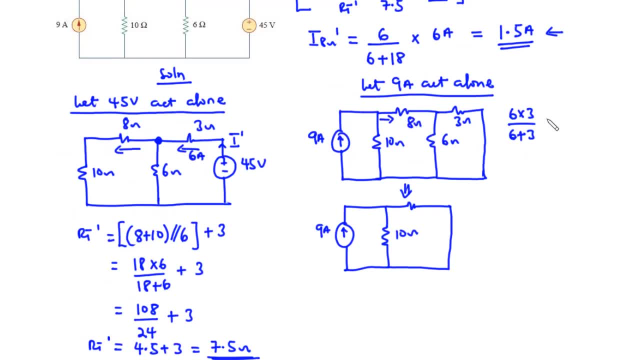 And then that will be in series with the 8 ohms resistor. So plus 8.. 6 times 3 is 18.. 6 plus 3 is 9.. So 18 divided by 9 is 2.. And then 2 plus 8 is 10.. 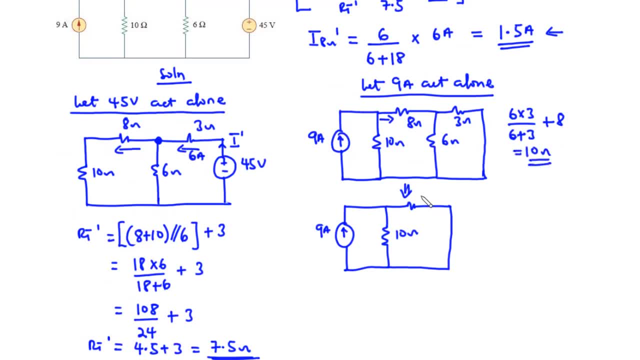 So we have 6.. So we have the combination to be 10 ohms. So we have 10 ohms here Now, since we have 9 amperes current moving to this junction And we have two resistors of the same value in parallel. 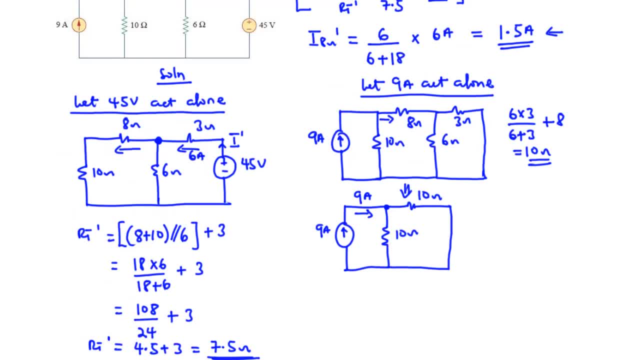 In that case, the current that is going to be distributed between the two is going to be half of the total current approaching the junction. So what this primarily means is that the current that is I8 ohm prime prime flowing through this branch and, for that matter, the 8 ohm resistor, is going to be 4.5 amperes. 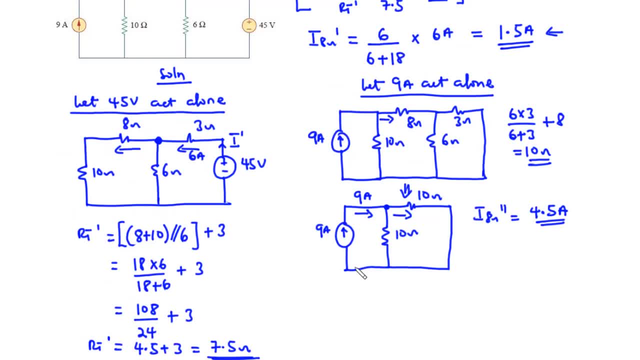 Which is half of the total current approaching the junction. Now, mind you, the current that flows through this branch, which is 4.5 amperes, is the same current that will be distributed between the 3 ohm resistor and the 6 ohm resistor. 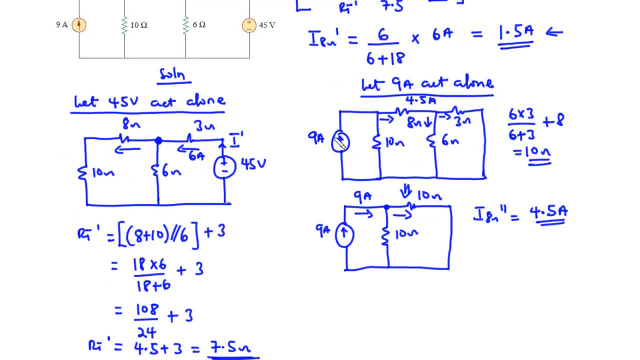 So the current that flows through the 8 ohm resistor When it is distributed between the 2 ohm resistor and the 6 ohm resistor, When the 9 amperes current is acting alone, will definitely be 4.5. 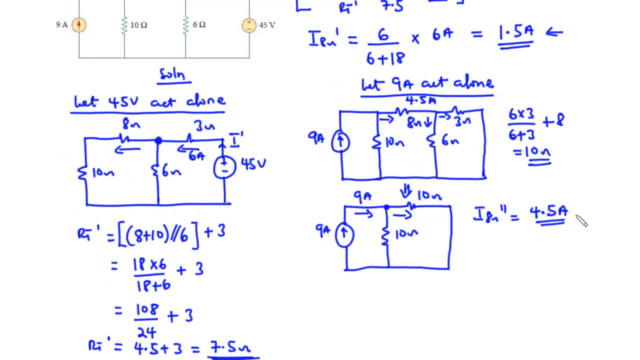 Now let's also note the direction of the current. It is moving to the right. So at this point we are going to add the two current values. Therefore we have I8 ohm equals I8 ohm prime, Plus I8 ohm. 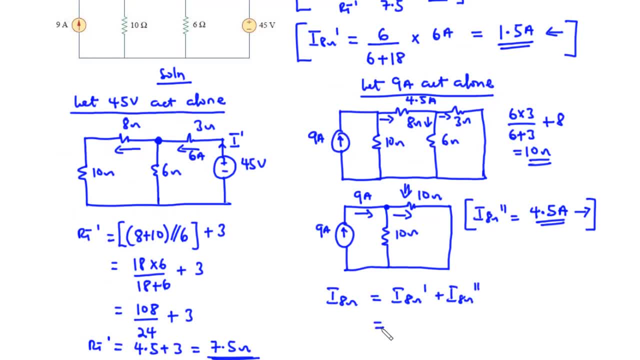 Prime. Now let's assume that the current moving to the left, That is, this current, is going to be a negative current, So that is negative 1.5.. And then the current moving to the right is going to be a positive current. 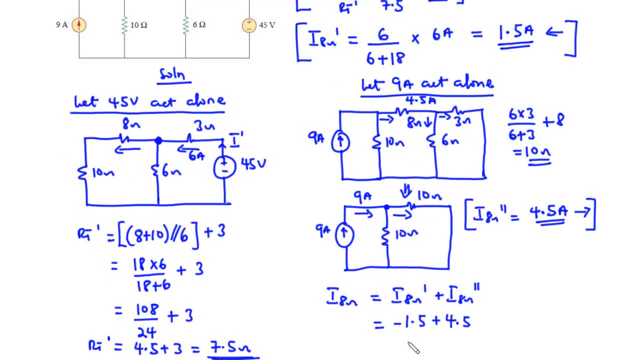 So we have plus 4.5.. Therefore, we have negative 1.5 plus 4.5 to be equal to 3.0.. So we have negative 1.5 plus 4.5 to be equal to 3.0.. 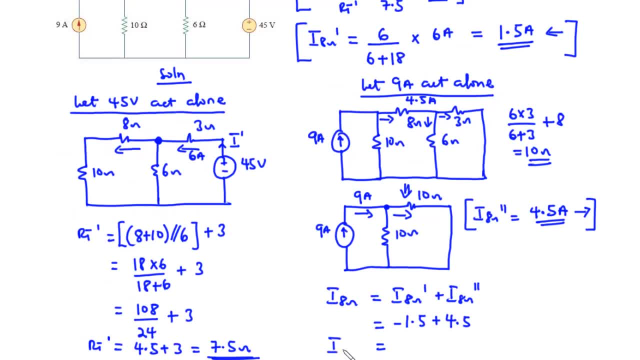 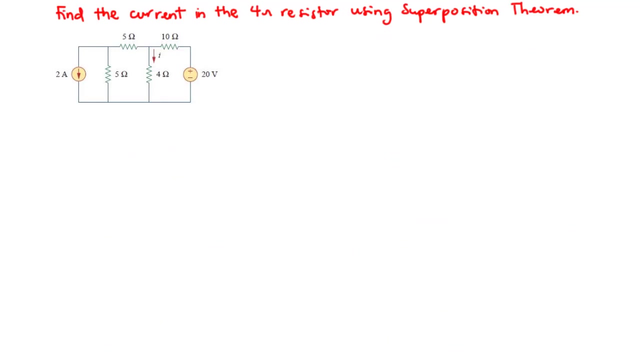 Therefore we have the total current flowing through the 8 ohms resistor to be 3.0 amperes. So basically, that is how to solve circuit problems using superposition theorem. Now let's move on to the next question. So for this question we are going to find the current in the 4 ohms resistor using superposition. 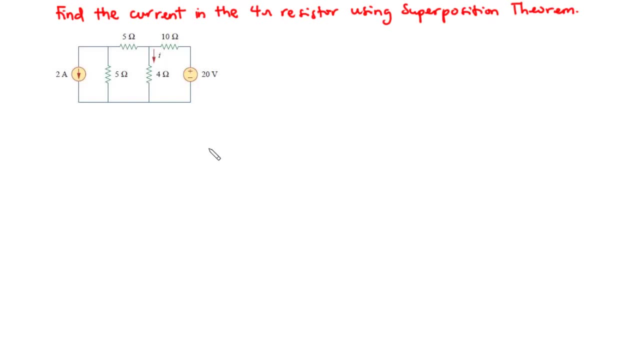 theorem. Now, from the previous question, We said that to solve a circuit using superposition theorem, The first thing we are going to do is to consider one of the sources acting alone while we deactivate the other source, And then we find the current flowing through the resistor in question while we note the 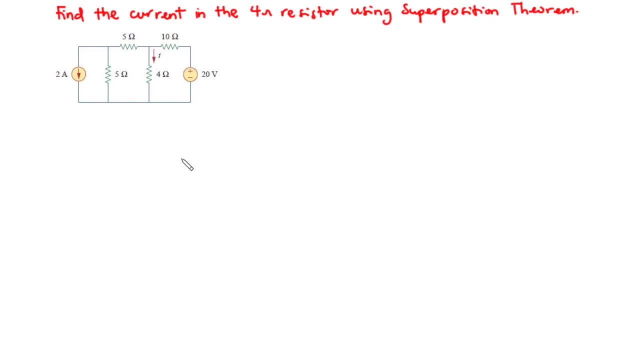 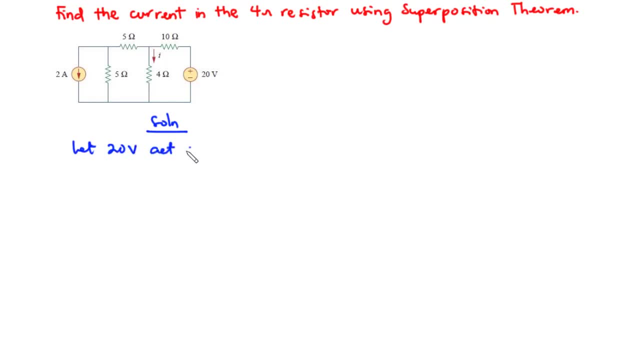 So let's consider the 20 volts acting alone. So let's consider the 20 volts acting alone, So theSimpleVolume dive valve, Which means that you are going to deactivate the 2 Amps current source And then we are going to replace that with an open circuit. 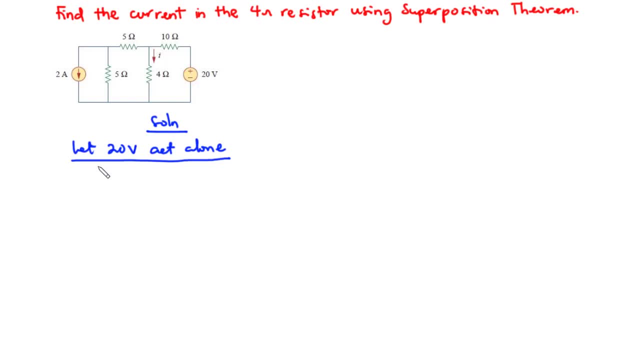 So let's redraw the circuit with the 2 Ampsenas source deactivated. This symbol on the right is the circuit function of the DC As sembler system. We can notice that does not apply on Ethernet. so we have this to be the 20 volts. we have 10 ohms, 4 ohms, 5 ohms and then 5 ohms. at this point 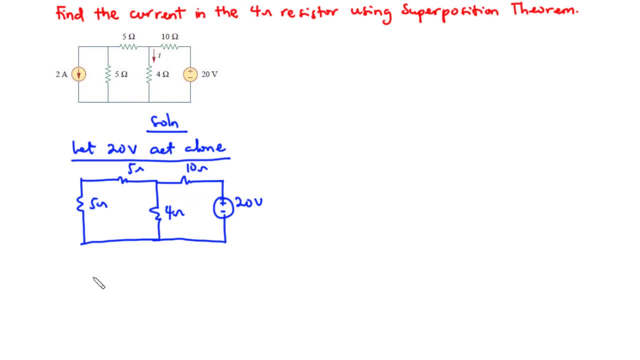 let's find the total resistance for this circuit. so we call that rt prime, and that is equal to: these two resistors are connected in series because we have the same current flowing through them and the combination is in parallel with the four ohms. and then all of that. 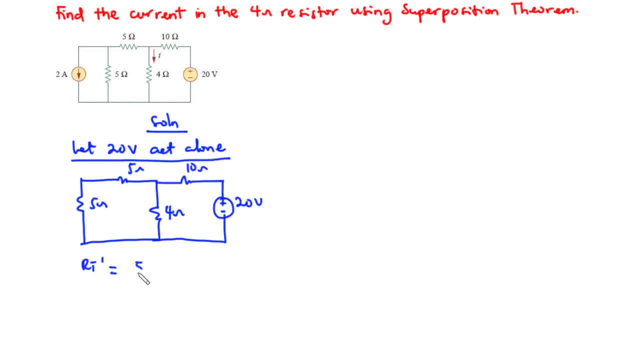 in series with a 10 ohms resistor. so we have 5 plus 5, all parallel 4, and then all of that in series with a 10 ohms resistor. so 5 plus 5 is 10. therefore we have 10 times 4 divided by. 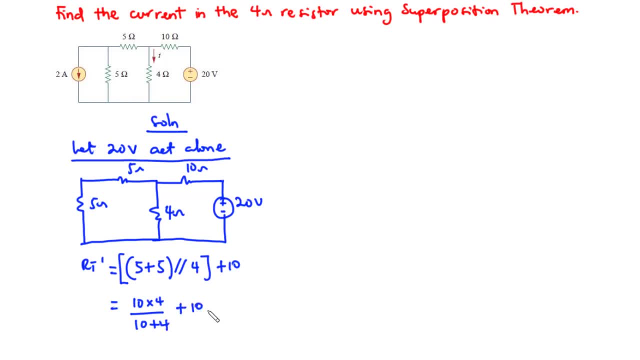 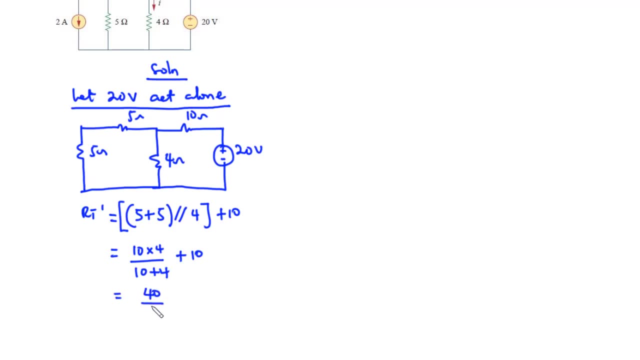 10 plus 4 plus 10, now 10 times 4 is 40, 10 plus 4 is 14, and then 40 divided by 14 gives 2.8571, and then plus 10 we have 12.8571 ohms. 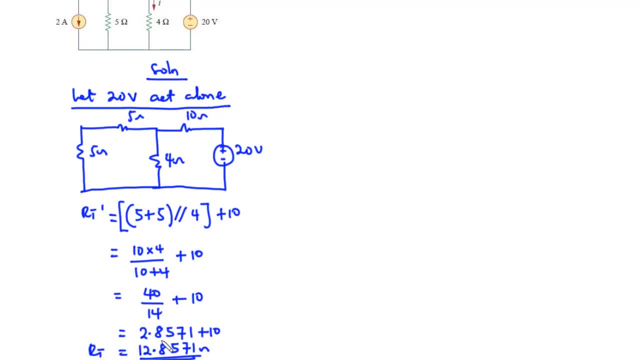 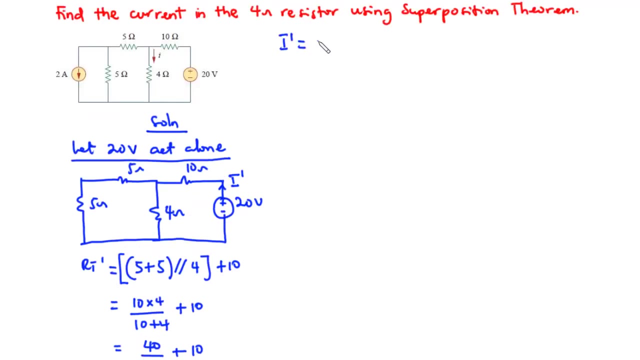 so this is the total resistance for this circuit. now let's find the total current produced by the 20 volts. let's call that I prime. so we have: I prime equals 20 divided by 12.8571, and that is equal to 1.5556 amperes. so that gives us 1.5550 amperes and as I mentioned earlier, this even shines along the string of current. and you also need to remember you have kind of better circuit for this issue known as magnetic field in general by now, but you can still use your conventional circuit like the PRC. but see, we can use normal circuit. that is because if you want aетр�� circuit and you need more of aетр느 spring current as an alternative for the techniques. you will need some more for the four ohms. so we have minus 5 times 4 volts and because we also have very low voltage, it takes us quite a lot of voltage from this. 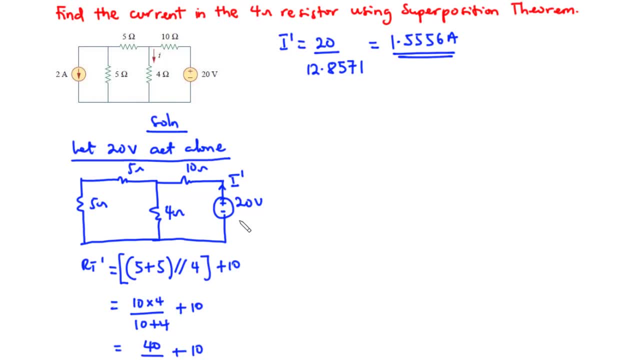 dot, but the problem is quite different because it talks about this until we register. So this is the total current produced by the 20 volts. Now let's find the current that is flowing through the 4 ohms resistor when the 20 volts is acting alone. 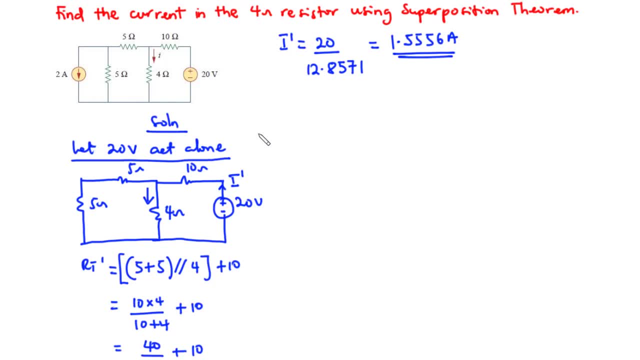 Now, in so doing, we are going to use the current division rule. So to find the current flowing through the 4 ohms resistor, let's call that I4 ohm prime. And that is equal to, because we are going to distribute current between the 4 ohms and the combination of these two resistors. 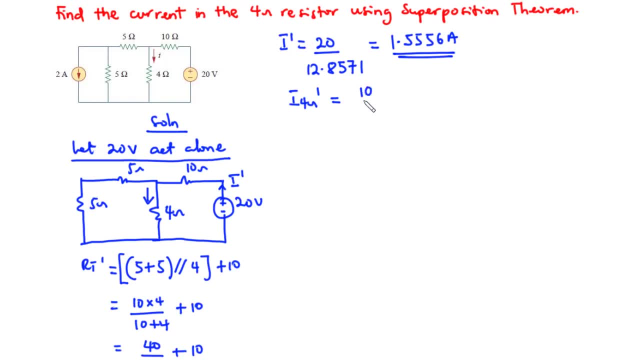 we have 5 plus 5, which is 10.. So we have 10 divided by 10 plus 4.. And then we multiply that by the total current approaching the junction, which is 1.5556 amperes, So we have I4 ohm prime to be equal to 1.1111 amperes. 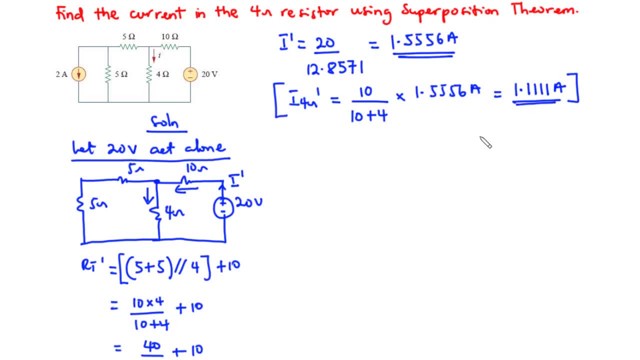 So this is the value of current that flows through the 4 ohms resistor when the 20 volts is acting alone. Now let's deactivate the 20 volts and then consider the 2 amperes current. So let 2 amperes act alone. 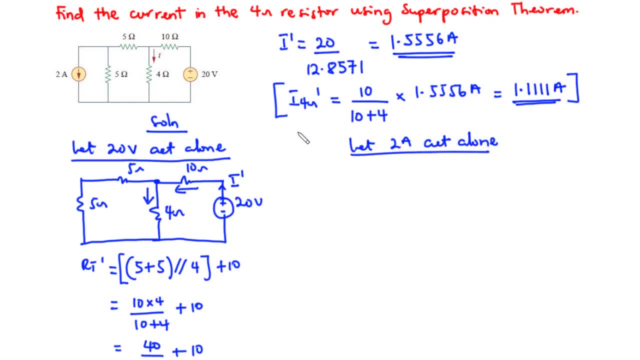 So let's redraw the circuit deactivating the 20 volts. We have this to be the 5 ohms resistor. We also have this 5 ohms resistor. We have this to be the 4 and the 10 ohms resistor. 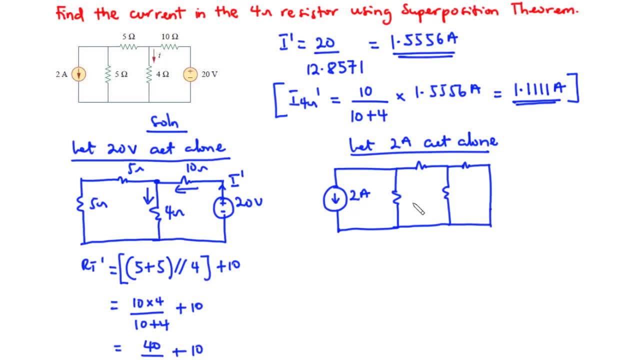 We have the voltage source short circuited. Now to find the current flowing through the 4 ohms resistor, we first of all need to combine these three resistors, So the 4 ohm resistor is in parallel with the 10 ohm resistor. 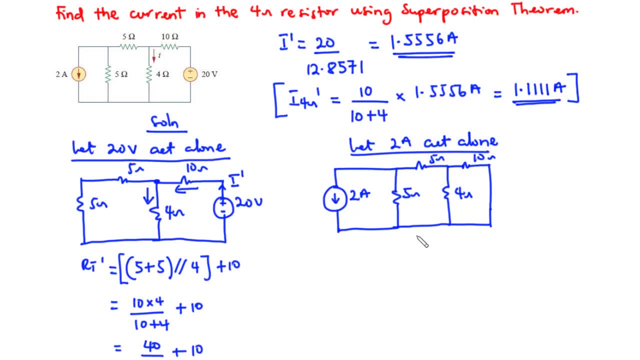 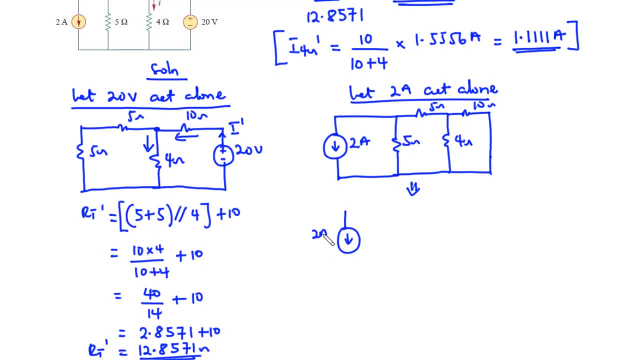 And the combination is in series with the 5 ohms resistor. So we can simplify this circuit so that it looks like this: We have 2 amperes And then we have 5 ohms And the combination of these three resistors here. 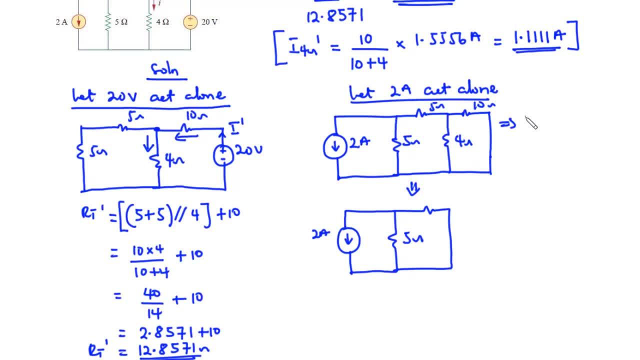 So we have 4 in parallel with 10, which is 4 parallel 10.. And then all of that in series with the 5 ohms resistor. Now we have 4 parallel 10 to be 2.8571.. So we have 4 parallel 10 to be 2.8571.. 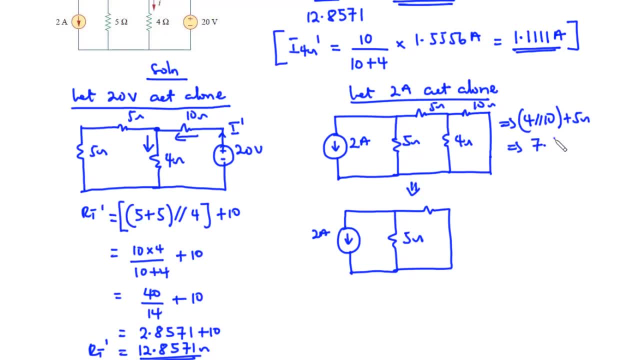 And then we have 4 parallel 10 to be 2.8571.. So plus 5 becomes 7.8571 ohms. So that is the resistor we have here, 7.8571 ohms. So we have this current flowing in this direction. 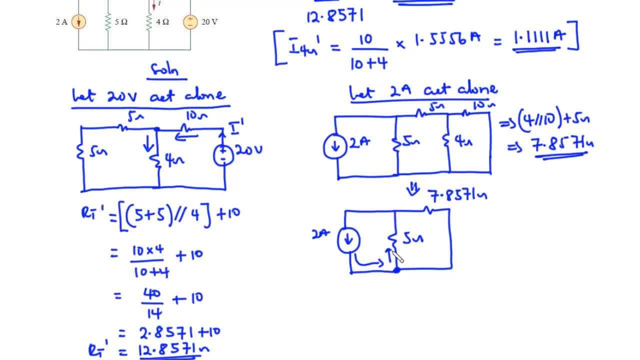